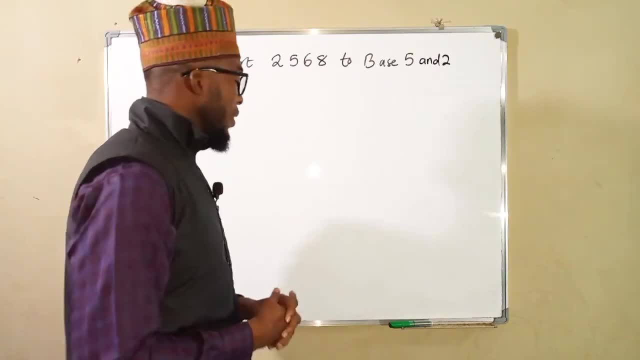 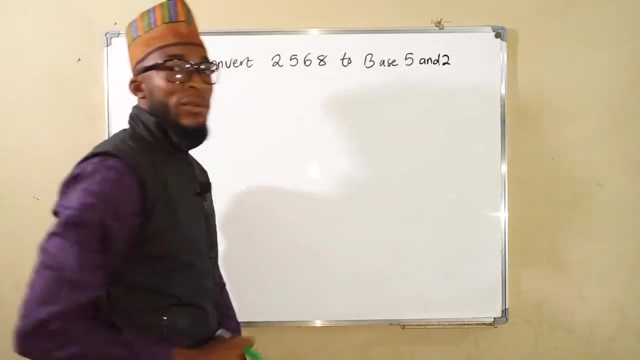 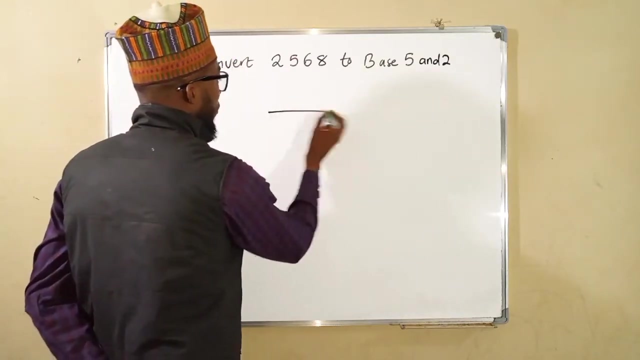 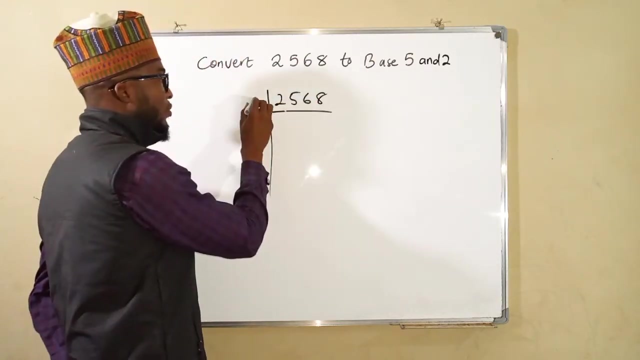 which means that it is in base 10.. To start with base 5, we are going to perform a successive division of this number with 5 and of 10,. the remainders are in their descending order. So this is 2,568.. We are going to divide through by 5.. 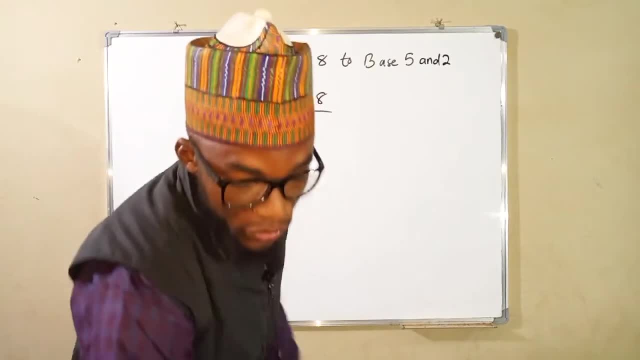 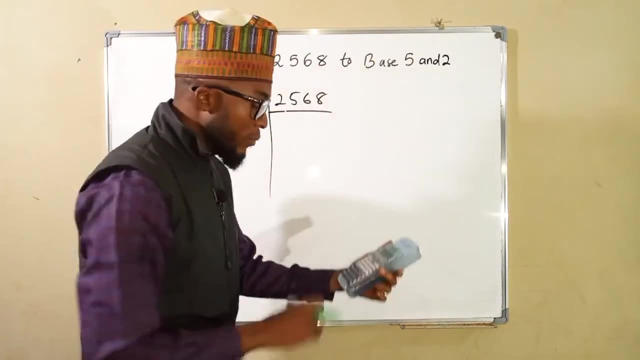 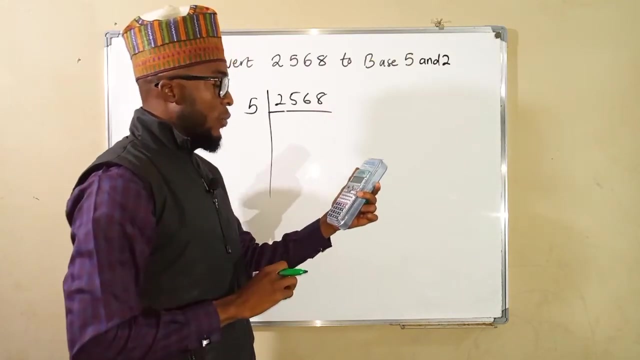 For convenience, we can use a calculator. So this is my calculator. I will divide the whole of these numbers by 5. And of 10, the remainder. So we have 2,568 divided by 5.. What I have here is 5,1,3.. Do not include the decimal number. 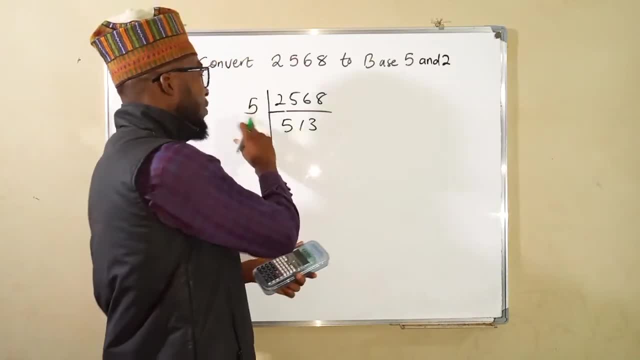 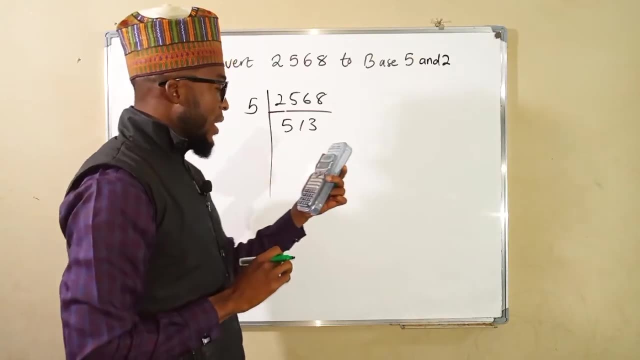 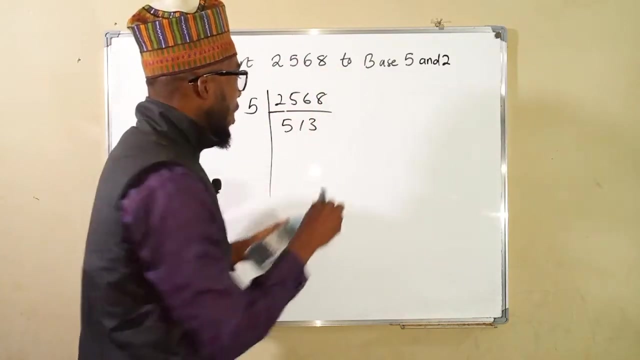 So this 5,1,3, you should multiply it with 5.. 5,1,3 times 5.. What I have here is 2,565.. But this one is 68. This means that we have a remainder of 3.. 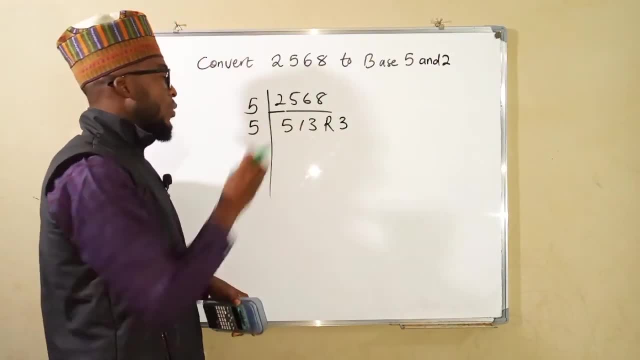 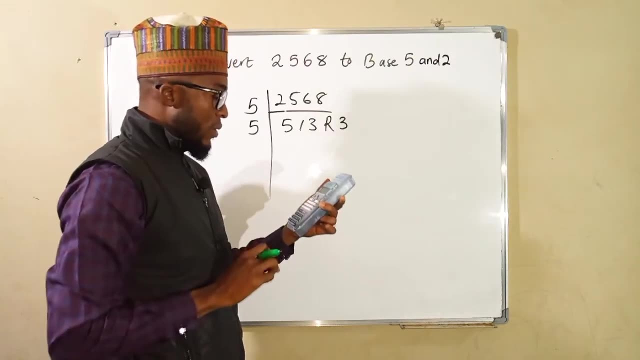 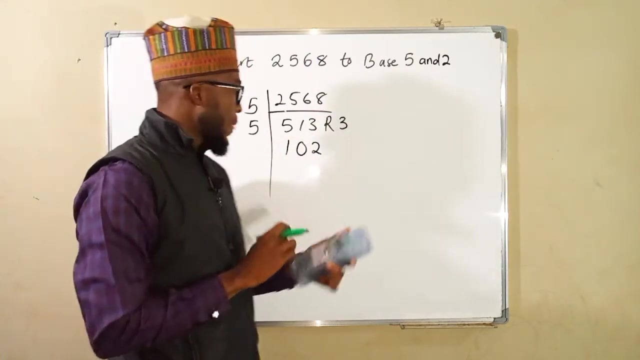 We continue. We divide this number by 5. again, 5 tightens divided by 5.. chance of dokłading a vitamin D. What I have here is 102.. To obtain the remainder, we say 102 times 5.. 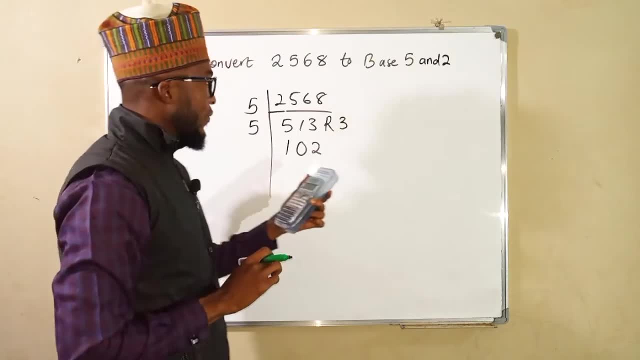 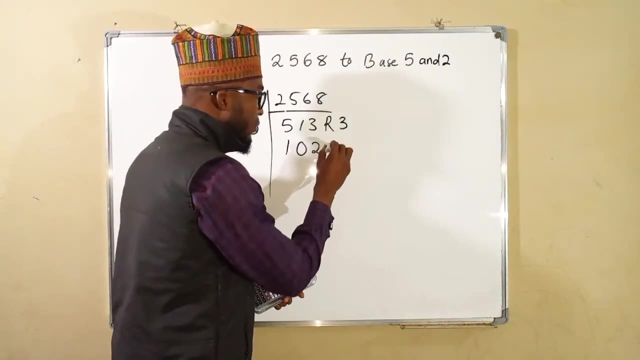 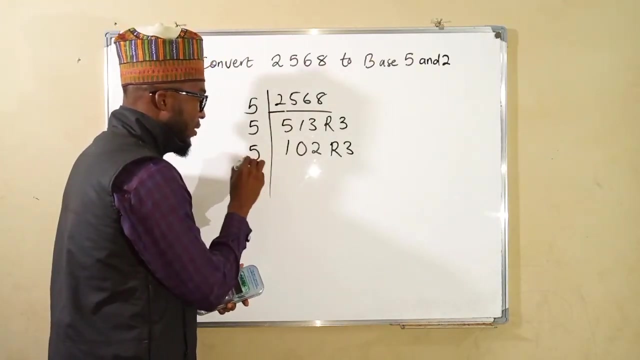 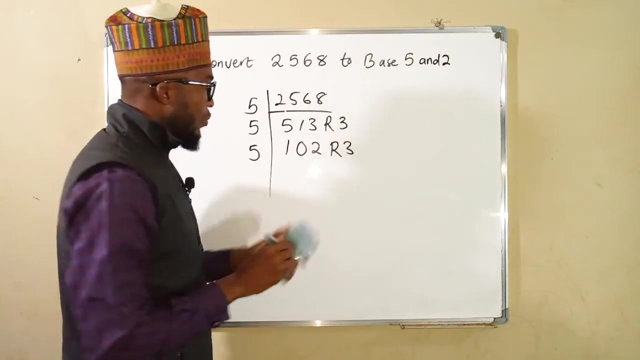 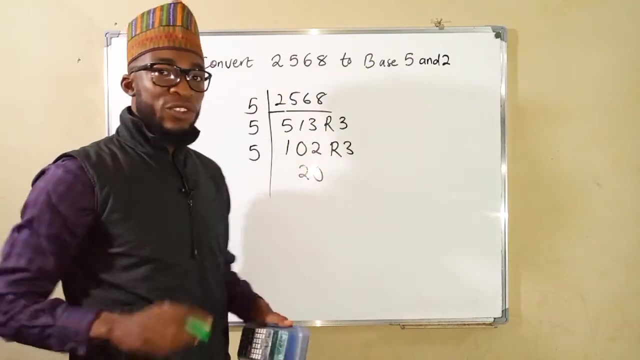 two times five, we have five hundred and ten. but this is five hundred and thirteen. this means that we also have a remainder of 30. we again divide 102 by five. one or two divided by five, what we have is 20. but if you times 20 by 5, you shall get 100. but 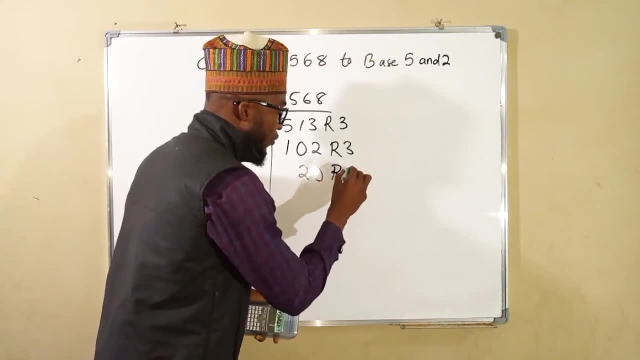 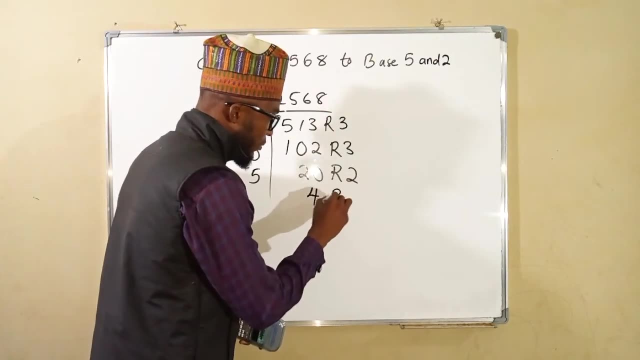 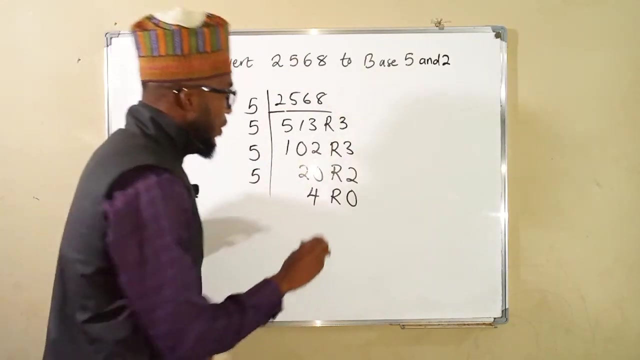 this is 102. this means that we have a remainder of 2.. 5 again. it can go into 24 times without remainder, without reminder, but 5 cannot longer go into 4, so we stop, we are going to do this again. so we have four, four times five, and we have a remainder of 3 and we are getting. 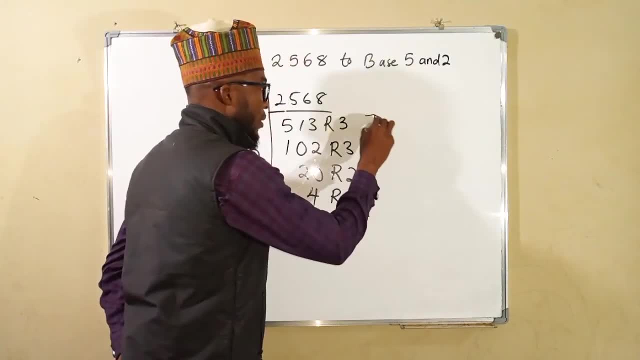 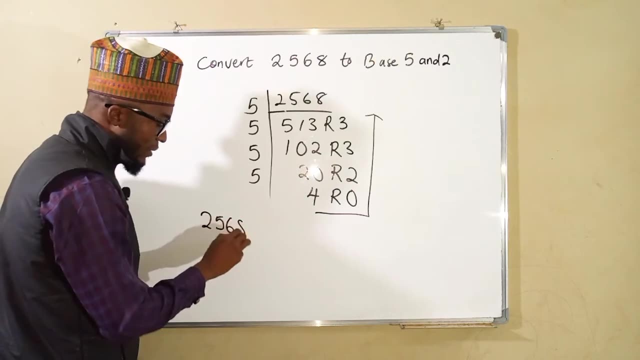 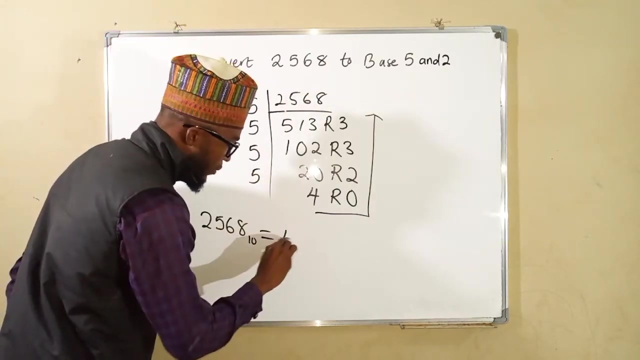 four times. we have a remainder of 3 and we are getting going to take these numbers in this form upward and conclude by saying two thousand five hundred and sixty eight, which is a number in base ten. this is the same thing as you start with this number: four, zero, two, three and finally, 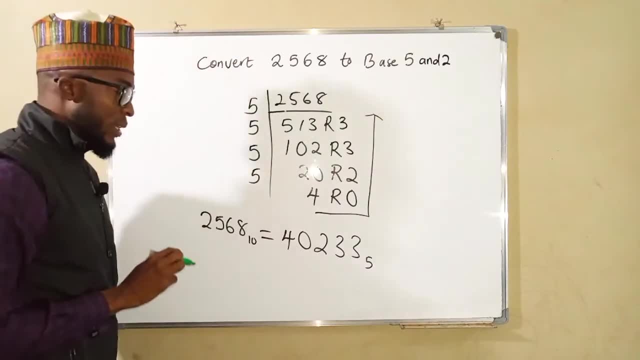 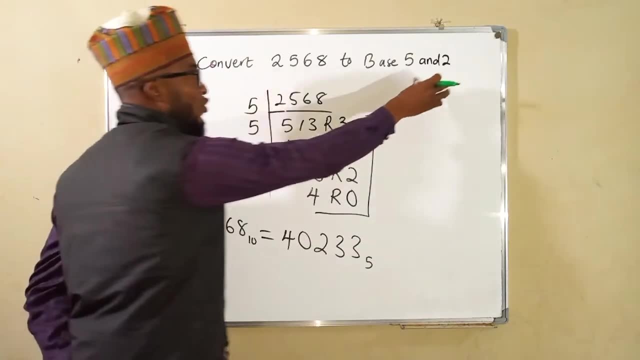 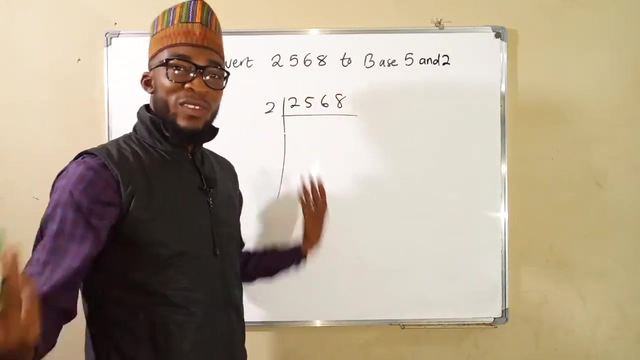 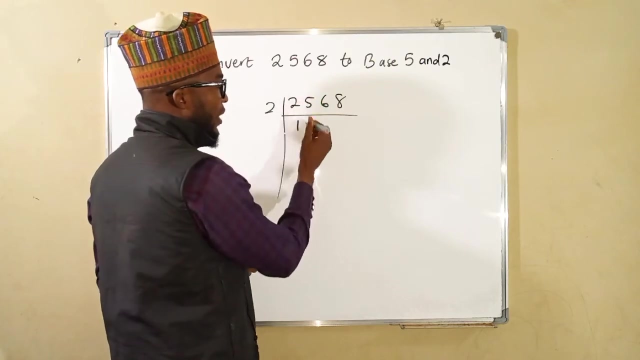 three, but this number is in base five. so they're exactly the same, just that they are in different bases. so now let us see how we can convert it to base two. so dividing numbers by two is the most simplest division, so we can even do it without calculator. two can go into two one. two can go into five two times. but 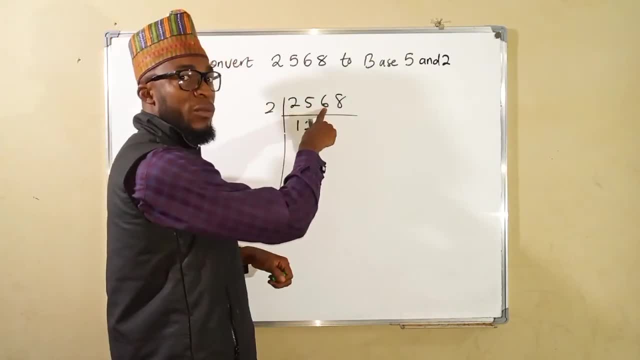 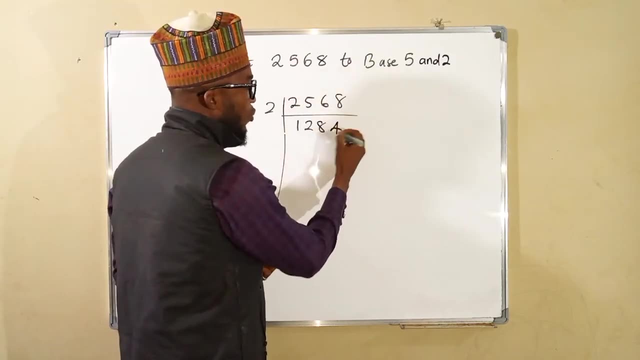 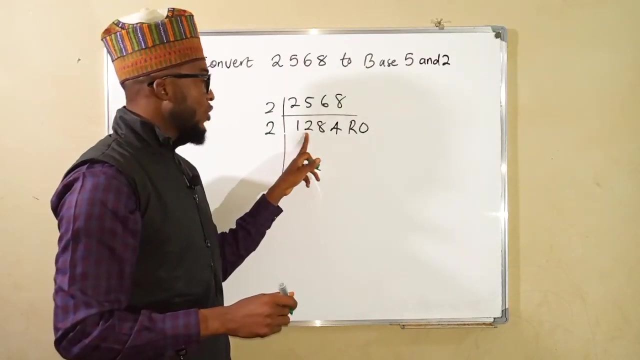 we have a remainder of one. take that one to the next number, it becomes sixty ten. two can go into sixteen eight times. two can go into eight four times. so we do not have any remainder. we move again two. two cannot go into one. therefore we join them together to become twelve. two can go into twelve six times two can go. 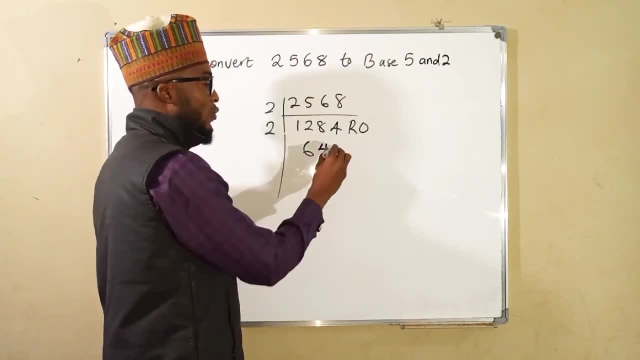 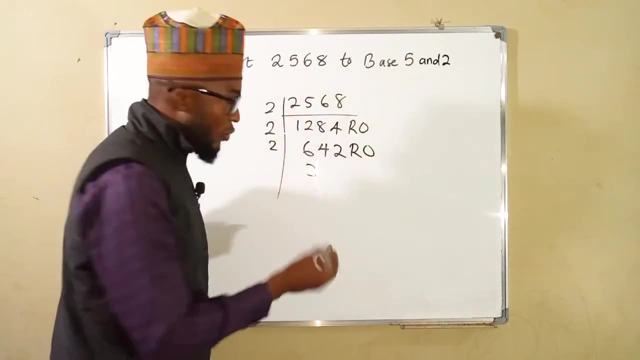 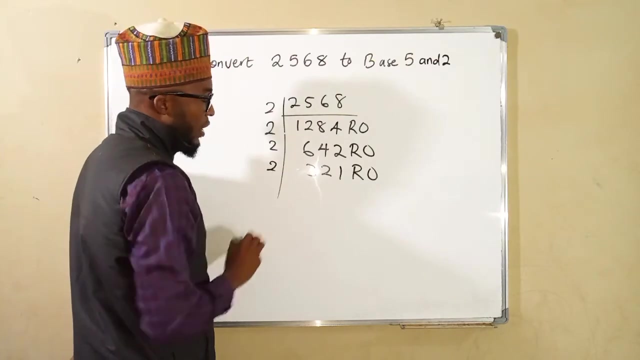 into eight four times two. can go into four two times, no remainder two again can go here three times. two can go into four two times two. can go into two one time without remainder two here. two can go into three one time, but we have one left. take that one to the next number. it. 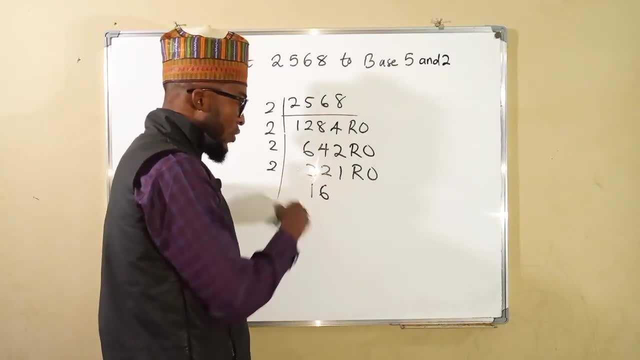 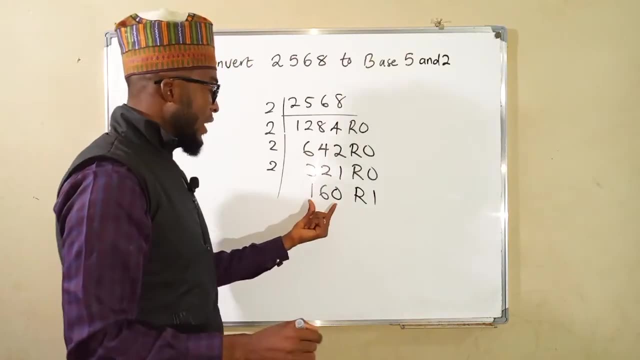 becomes twelve. two into twelve. six two cannot go into one, so we write zero. but we have one left, because if you times 160 by 2, you shall get 320, so we have one left. so we have one left, because if you times 160 by two, you shall get 320, so we have one left. 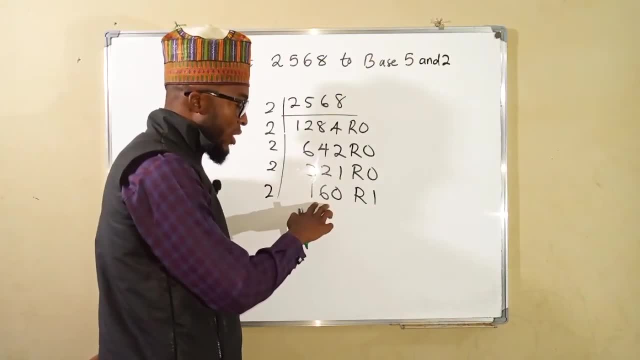 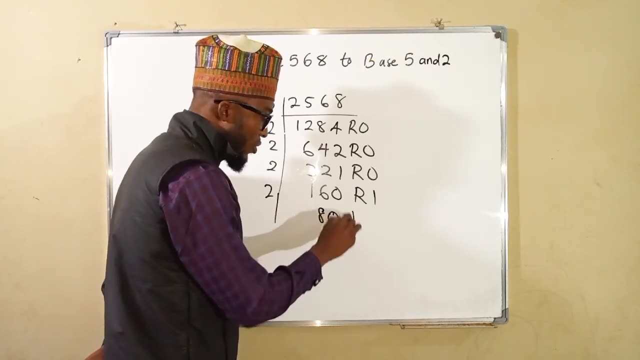 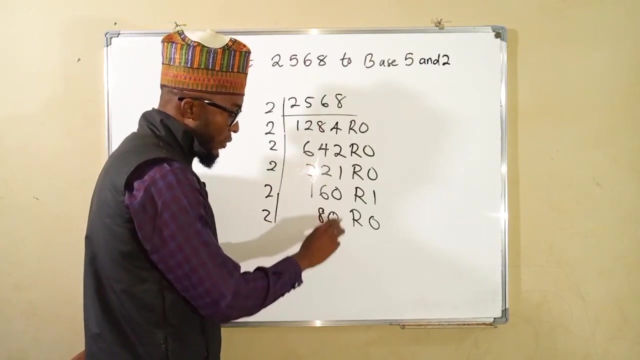 Again, 2.. 2 cannot go into 1.. You join them together. 2 can go into 16. eight times 2 into 0 is 0.. We do not have a remainder 2 here, we have. 2 into 8 is 4.. 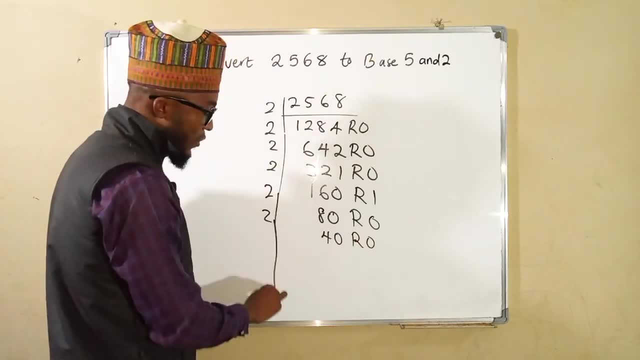 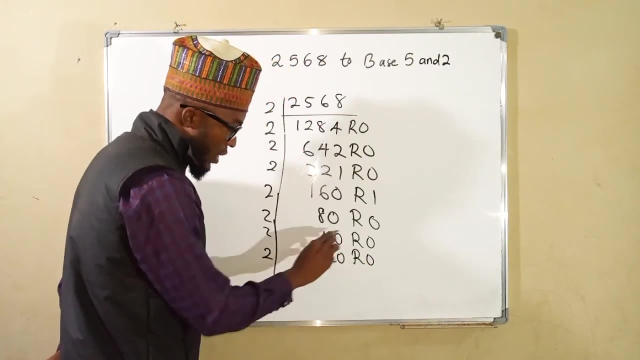 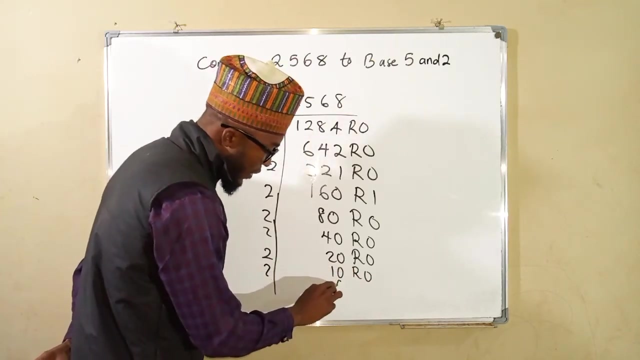 Here we have 0.. No remainder, We keep on going. 2 here we have 20.. No remainder. 2 here we have 10.. No remainder. 2 here we have 5.. No remainder. 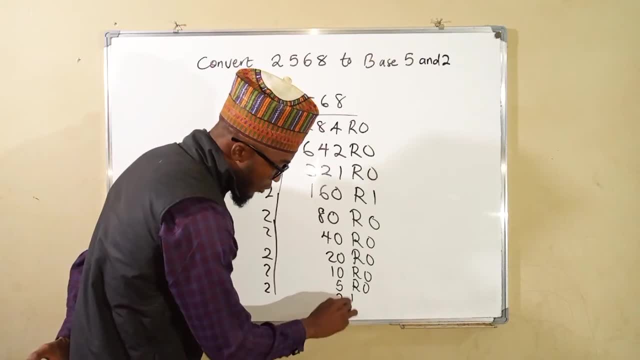 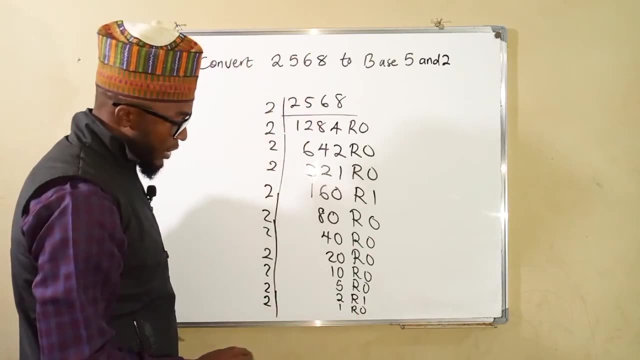 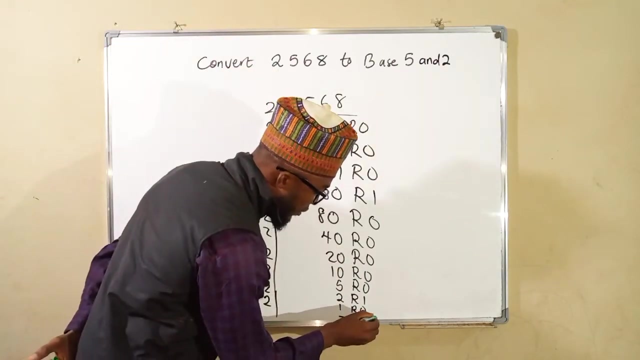 2. here we have 2.. But we have a remainder of 1.. 2 into 2 is 1.. No remainder. And finally, 2 cannot go into 1.. Therefore, we stop And take these numbers in this form. 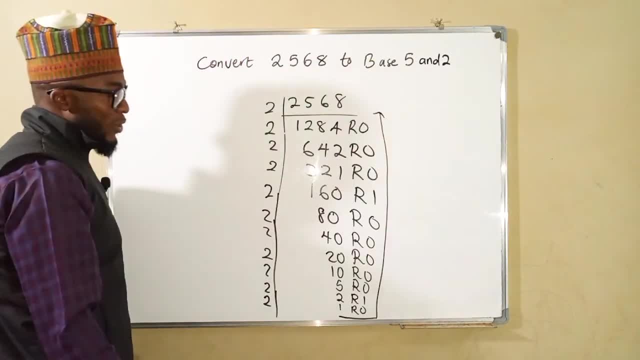 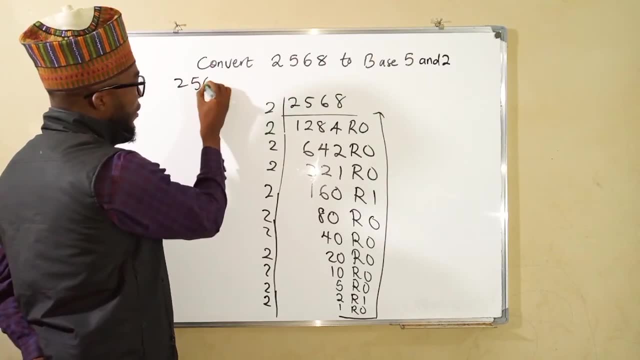 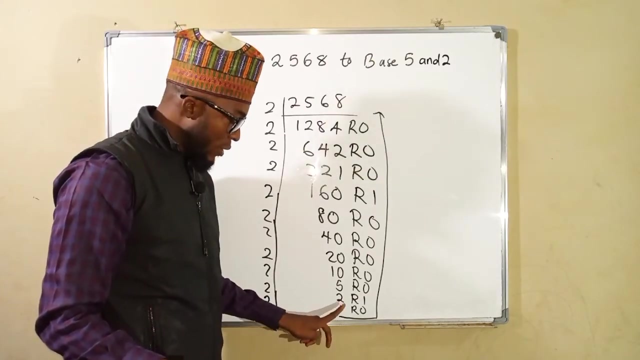 So where are we going to write them? Let me write them here: 2,, 5,, 6,, 8 is a number in this thing. It will be equal to. We start with this number here, which is 1.. 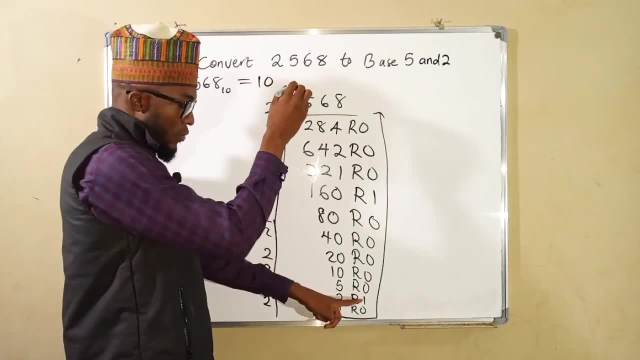 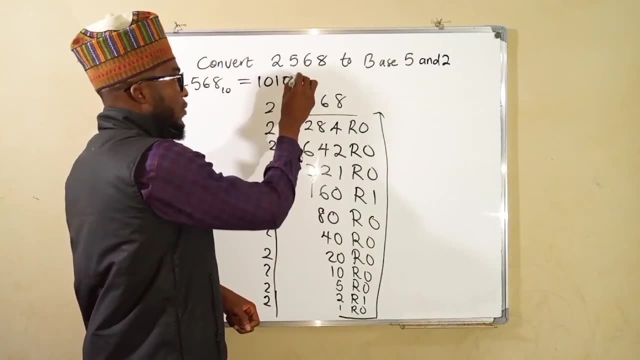 Then we move to the right. We have 0.. We have 1.. Then we have 0s- 1,, 2,, 3,, 4, 5.. 1,, 2,, 3,, 4, 5.. 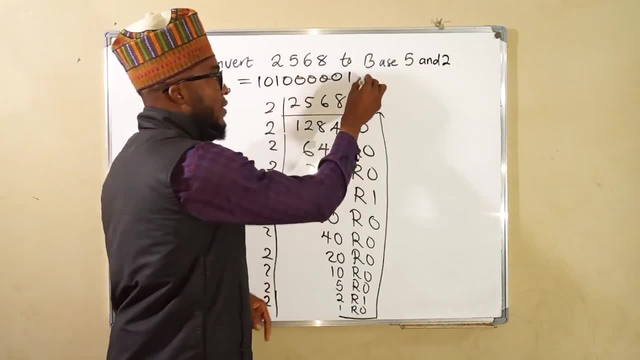 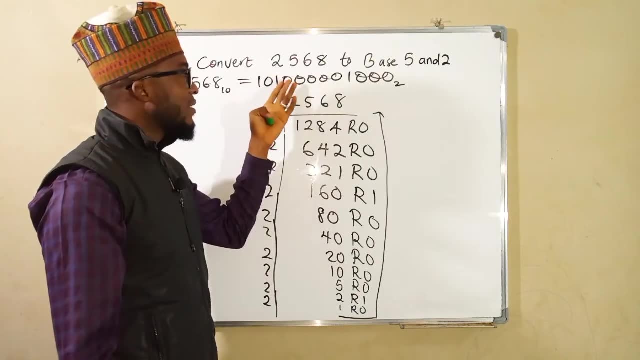 Then we have 1.. Then we have 3 other 0s, But this number is in base 2.. Remember I told you, the highest digit in any number base is 1 less than the base. This is why we do not have 2 here. 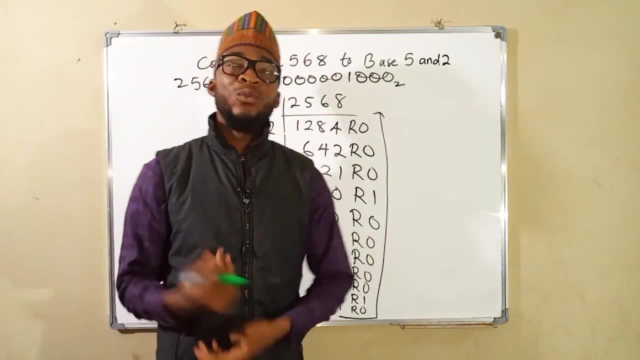 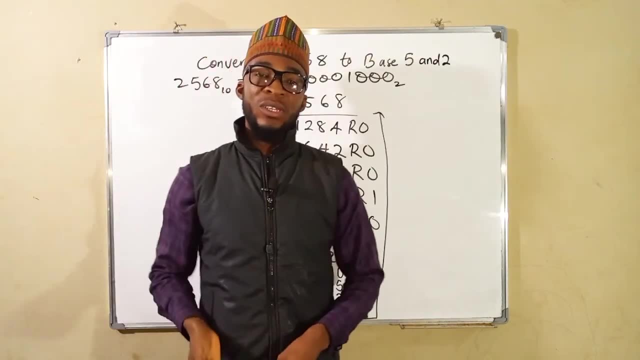 We do not have 10 here, So in our next class we shall see how to convert numbers in base 10 that are in decimal form to other bases. Thank you, Thanks for watching. Do have a nice day.